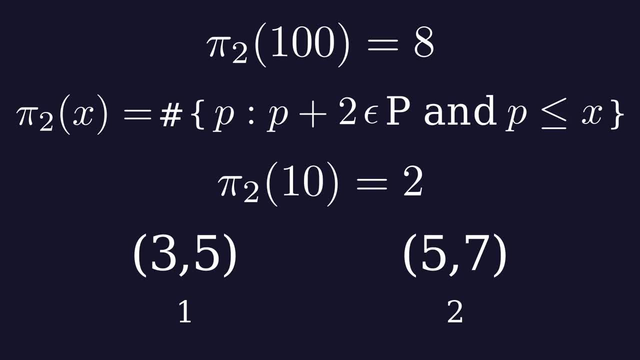 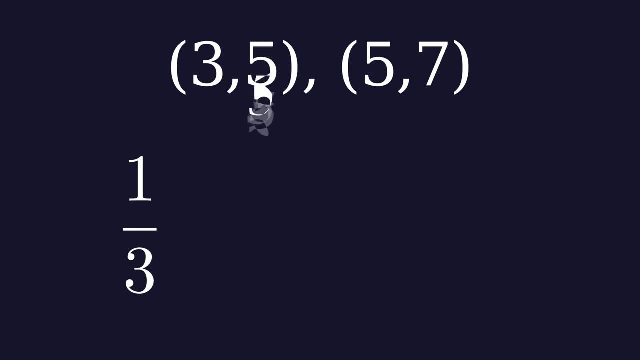 us an idea of how frequent or rare twin primes are, as x increases. Another way to measure the density of twin primes is to look at their reciprocals. That is, instead of counting how many twin primes there are up to a certain limit, we can add up their inverses, For example the sum of the reciprocals. 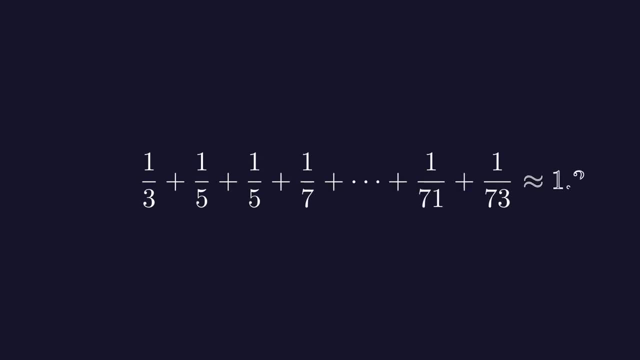 of the twin primes up to 100 is equal to around 1.33.. We can denote this sum by s2 of 100, where s2 of x is the function that sums the reciprocals of the twin primes with the smaller at most, x In general. 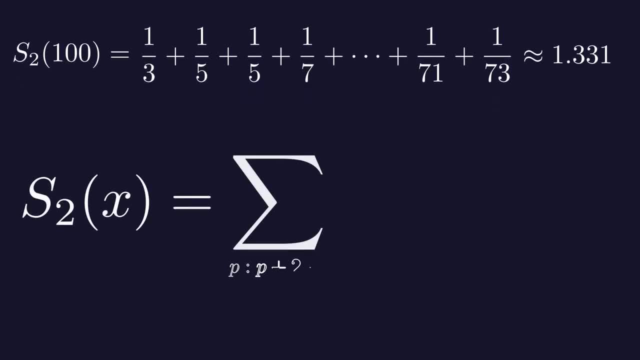 we can write s2 of x as the sum of all prime twins, where the capital P is the set of prime numbers. The function s2 of x gives us another idea of how frequent or rare twin primes are as x increases. But what happens if we let x go to infinity? Does s2 of x converge to a finite value? 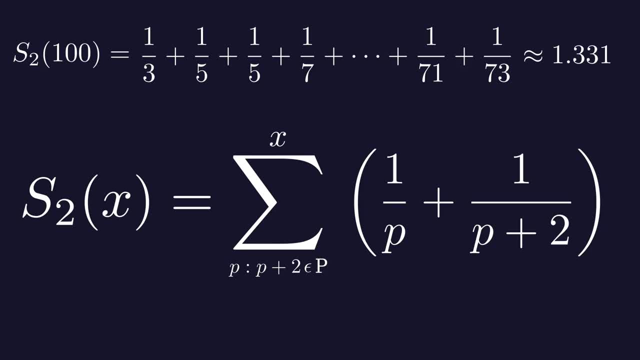 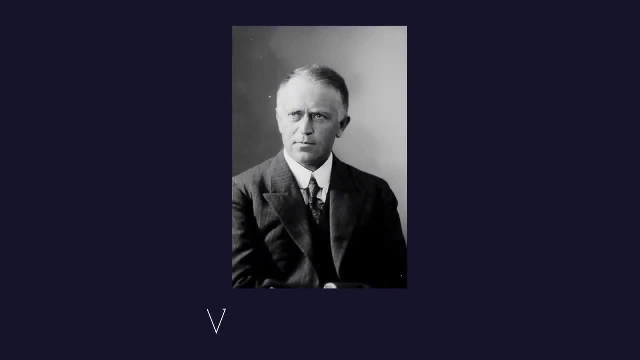 or does it diverge to infinity? And if it converges, what is its limit? The answer to the question of whether s2 of x converges or diverges was given by Viggo Brun in 1919.. He proved that s2 of x converges to a finite value as x goes to infinity. This means that the sum of 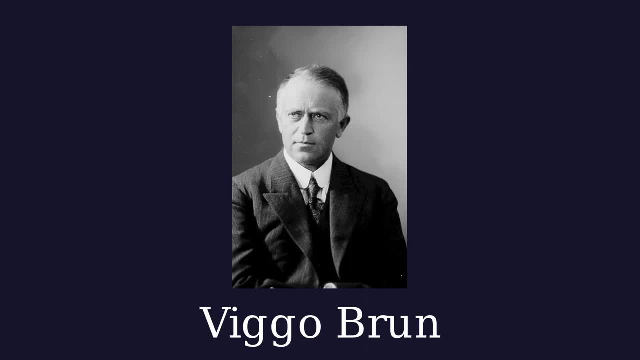 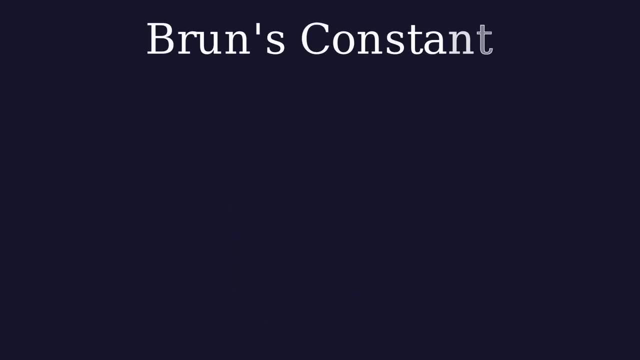 the reciprocals of all twin primes is a well-defined number, even though there may be infinitely many twin primes. This number is called Brun's constant and it is usually denoted by p2.. In other words, we can write b2 as limit as x goes to infinity. 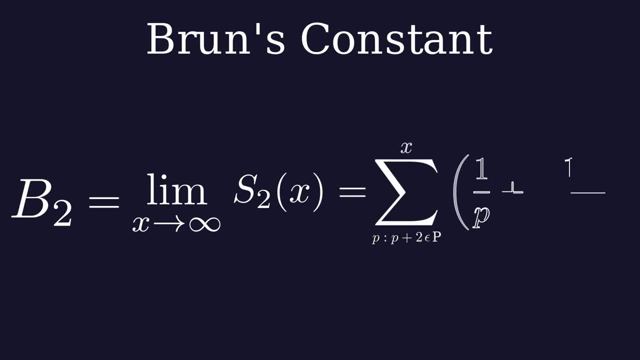 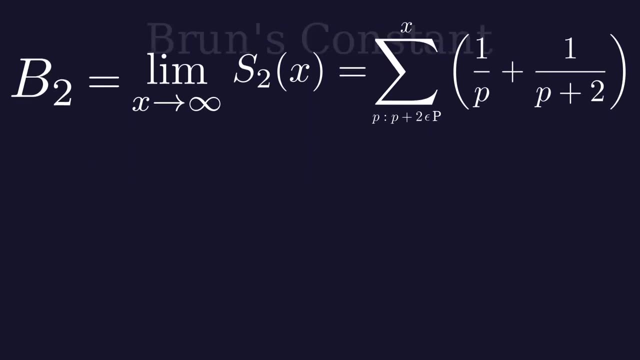 approaches infinity of s2. The exact value of b2 is not known and it may be irrational or even transcendental. However, we can estimate b2 by computing s2 for large values of x using computers and algorithms. The computation of b2 is not an easy task and it requires a lot of time and resources. The 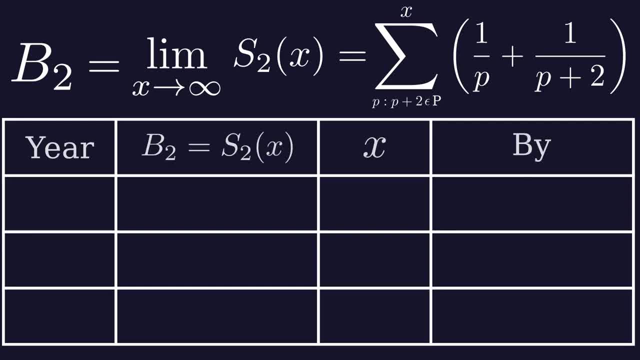 first person to estimate the Bern's constant was Brun himself, who used all the twin primes up to 2 million and obtained b2 equal to around 1.9.. Later, other mathematicians improved this estimate using more twin primes and better methods. For example, in 1976, Richard Brandt used all the twin primes.